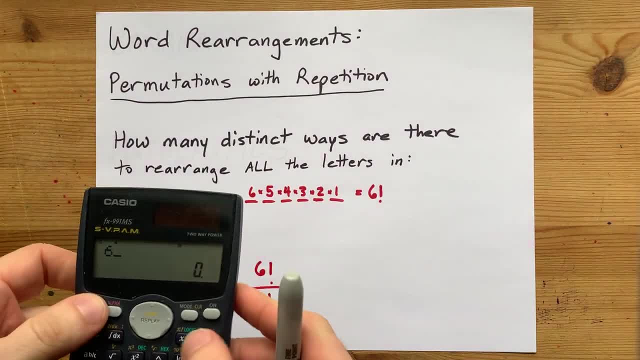 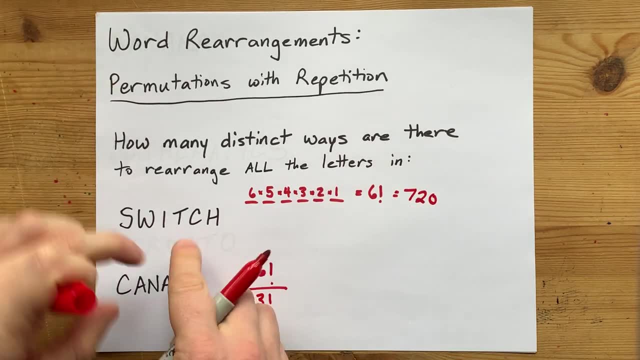 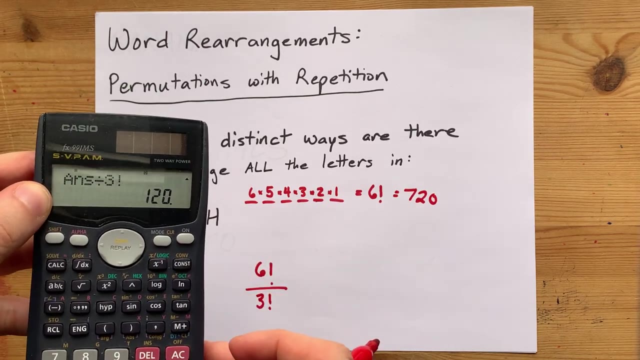 Now I'm going to do a little bit of math here. Six factorial on this calculator, Well, and yours too, is seven hundred and twenty. So there's seven hundred and twenty ways to rearrange this six letter word, But I have to divide by three factorial. 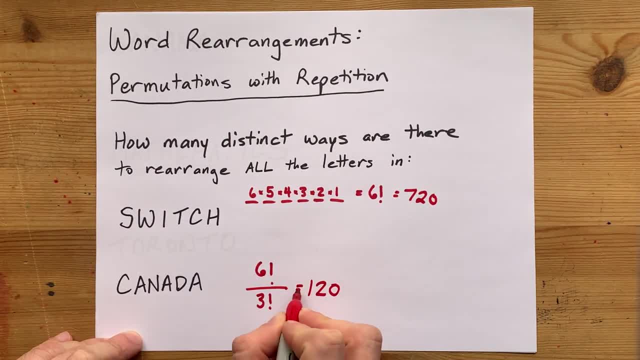 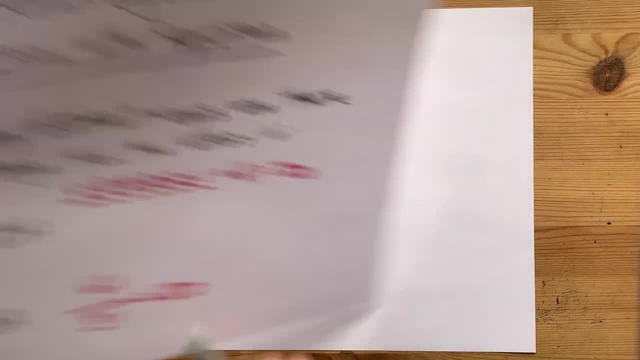 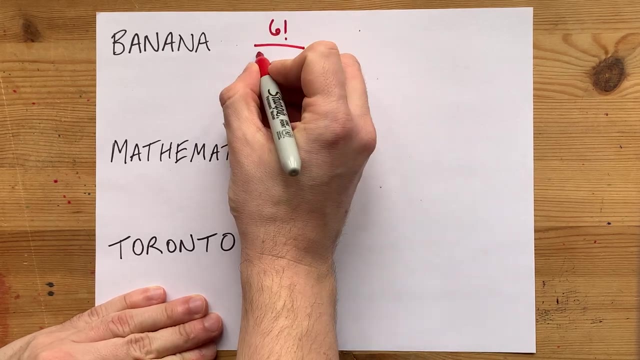 To get only one hundred and twenty distinct ways to rearrange the letters. here Again, I am dividing by three factorial for the three equivalent A's. Now let's just practice that together. Here we have a six letter word, Six factorial, And you divide by three factorial for the three A's. 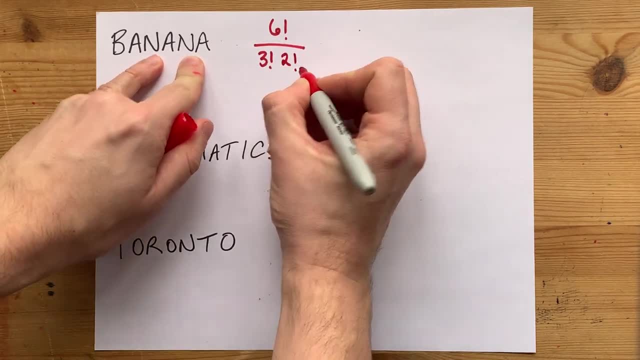 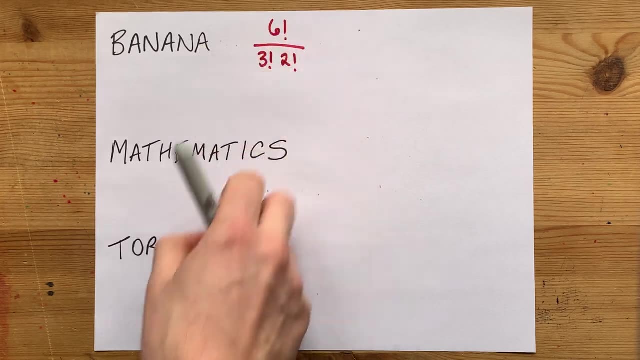 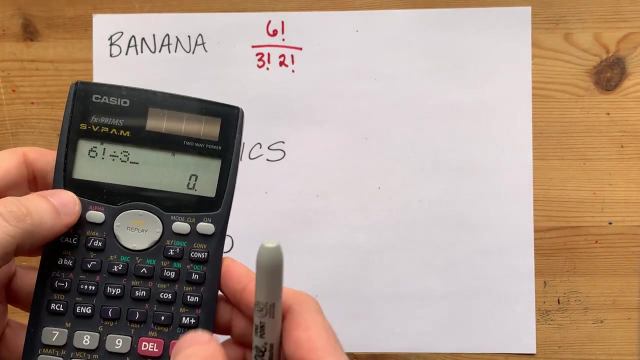 But you also have double ends. So you're going to divide by another two factorial. Now these are multiplied together in the denominator before you divide. But the other way to do that on your calculator is to type the top six factorial and you divide by three factorial for the A's. 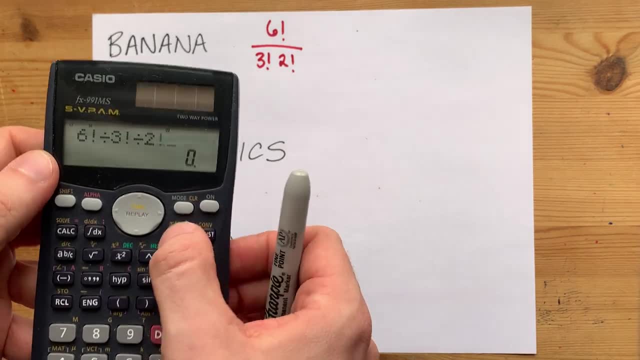 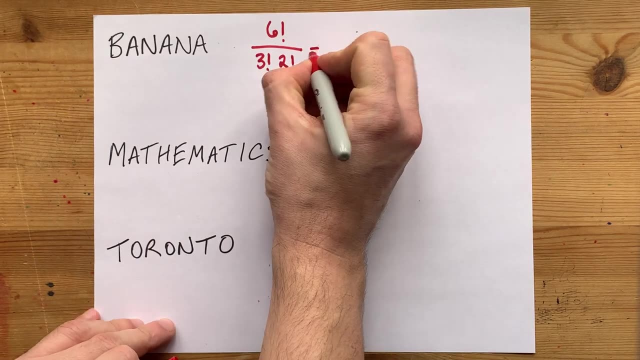 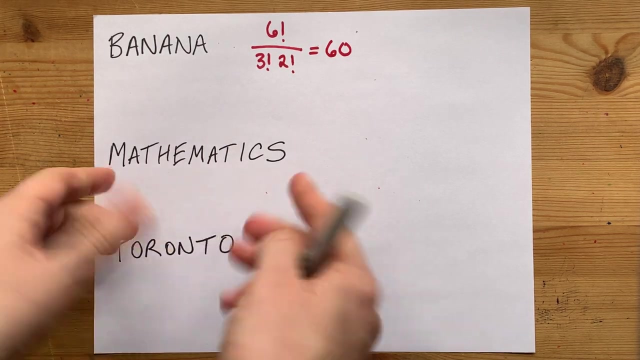 And then you divide again by two, factorial for the ends. So when you have three A's, two N's and a B, there's really only sixty ways to rearrange those six letters. Cool, Let's do the word mathematics, because some teachers love that word. 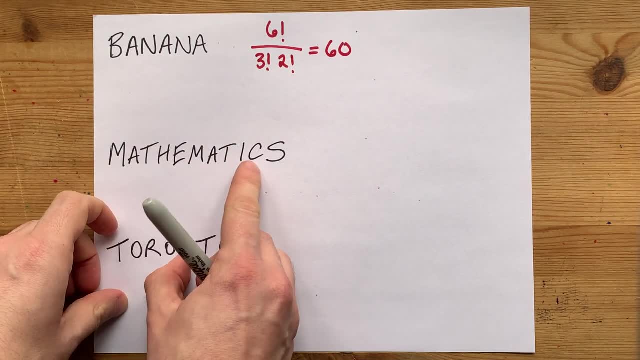 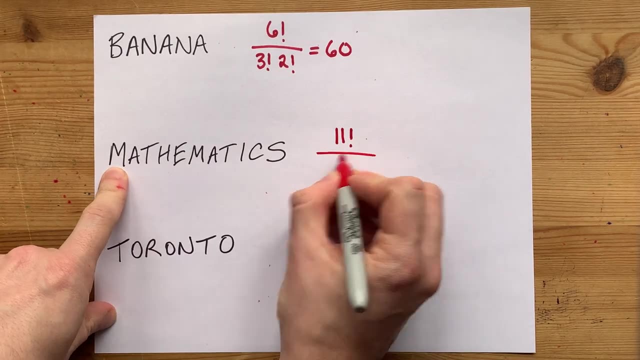 One, two, three, four, five, six, seven, eight, nine, ten, eleven letters, So that's eleven. factorial. in the numerator I have two M's, So I need to divide by two. factorial I have two A's. 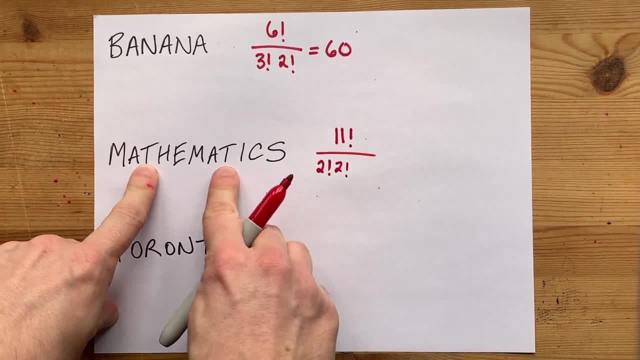 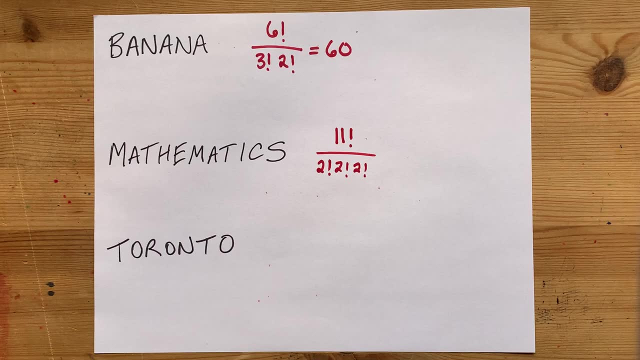 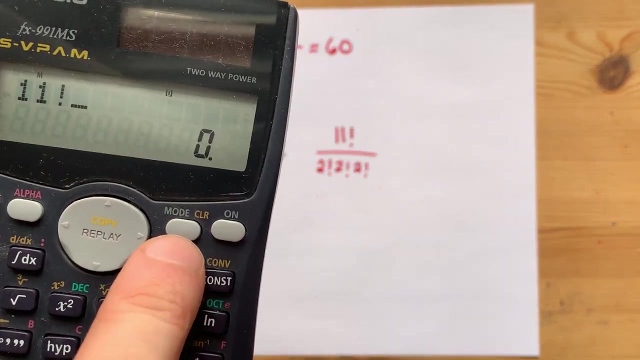 So I have to divide by another two factorial, Two T's, That's another two factorial, And all the rest of the letters aren't duplicated. So we just have to do eleven factorial. Now again on my calculator here I have a factorial button, this exclamation mark. 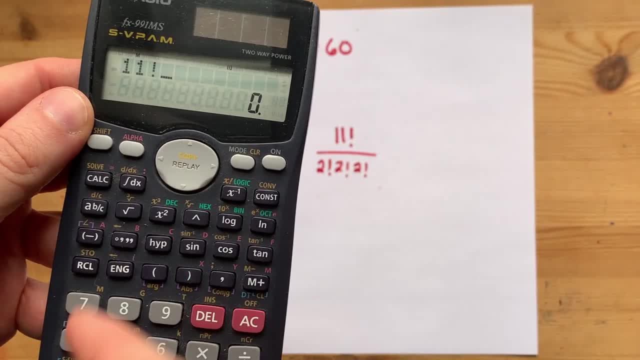 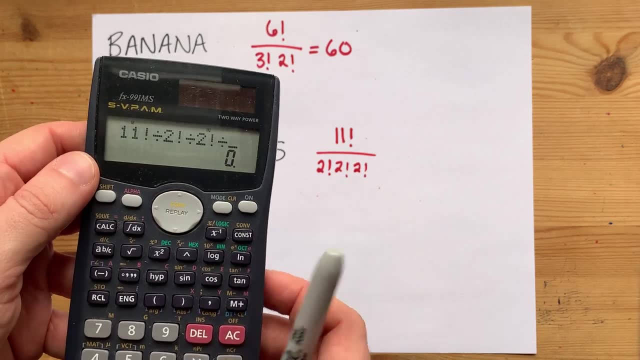 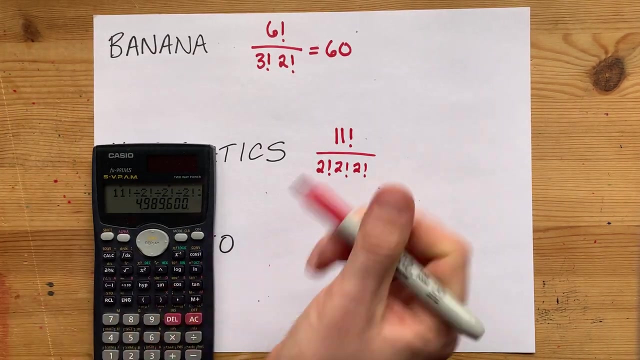 Surely you do as well. It's probably N factorial or X factorial, like mine, Divided by two factorial Three times. we're dividing by two factorial M's, A's and T's. Oh, that's still a large number. I get four million nine hundred and eighty nine thousand six hundred.